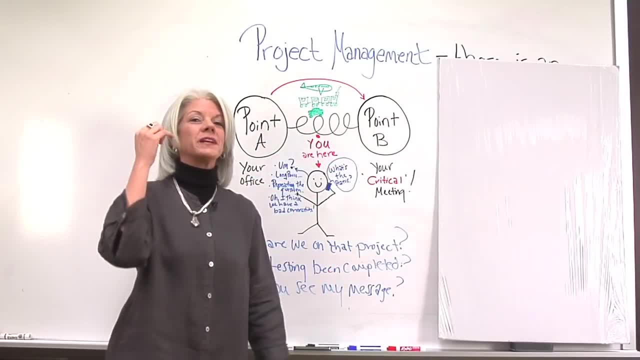 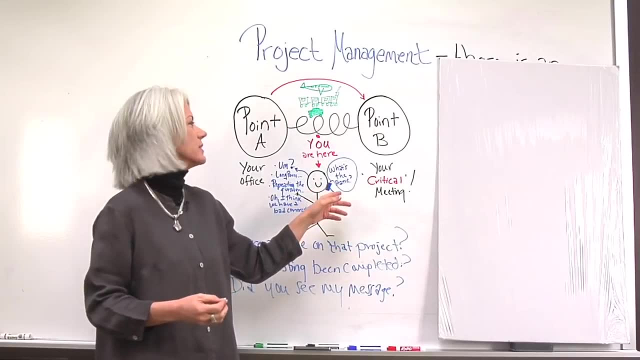 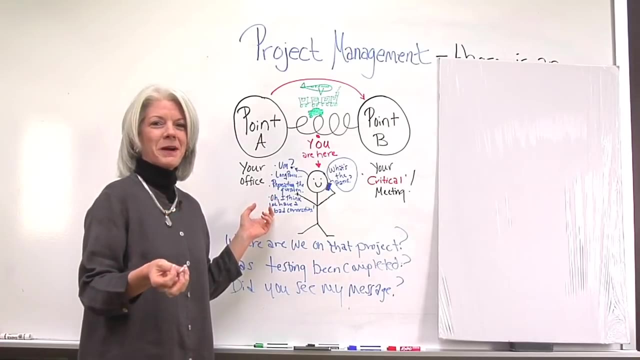 And you find yourself here And then what happens? You get the call. You get the call from your stakeholders or project team members or someone asking you that question. What's the status? And maybe some of your. if you're like me, sometimes some of my responses are: 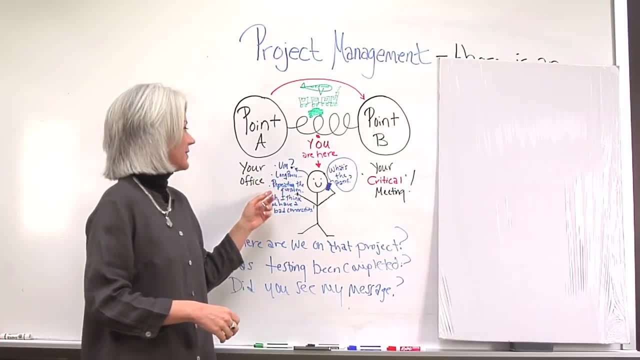 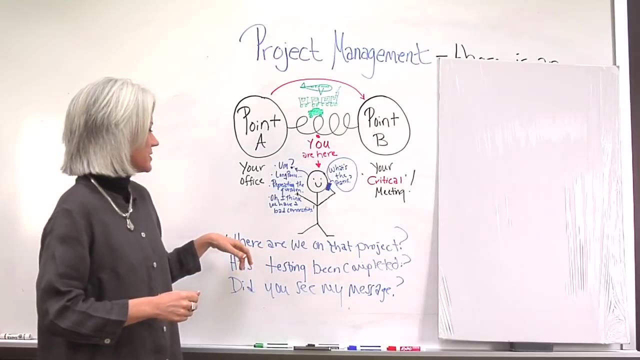 um, or I give a really long pause, or maybe a tactic is repeating the question, or even if things are really tough, um, I think we're having a bad connection And then the phone disconnects. Well, if you're looking, if you get these questions, where are we on that project? 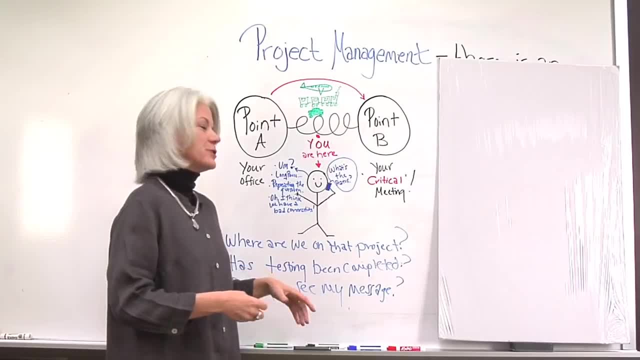 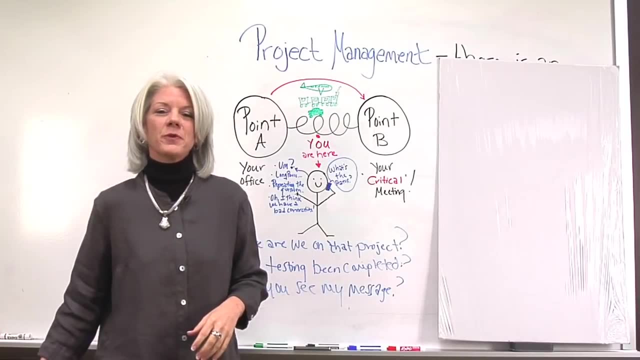 How was testing? Has it been completed? Did you see my message? If you get questions like this while you're trying to get from point A to point B, then if you're looking for a better response than these- um, sometimes I find myself trying to fumble through my book. 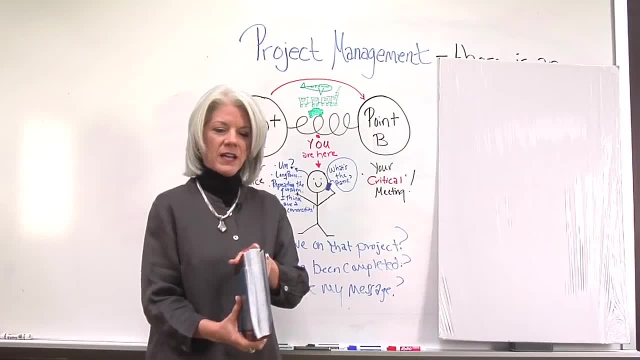 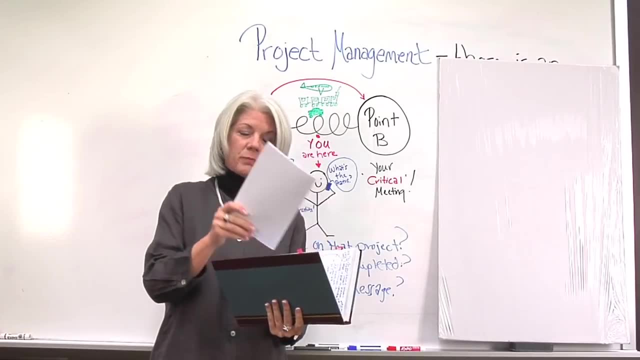 Maybe I'm literally in an airport and I'm trying to find. maybe maybe I printed out some- uh, a project plan, or maybe I made some notes in my book, so I'm trying to get to a plane or a flight on time. 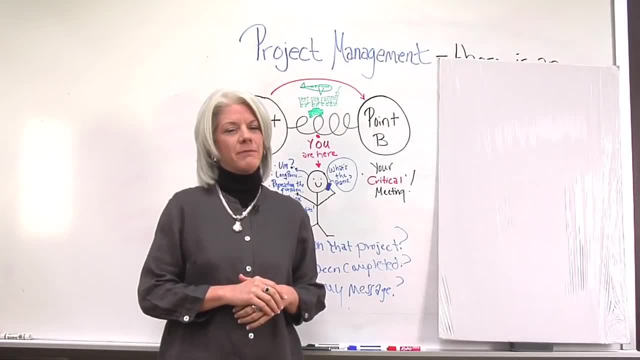 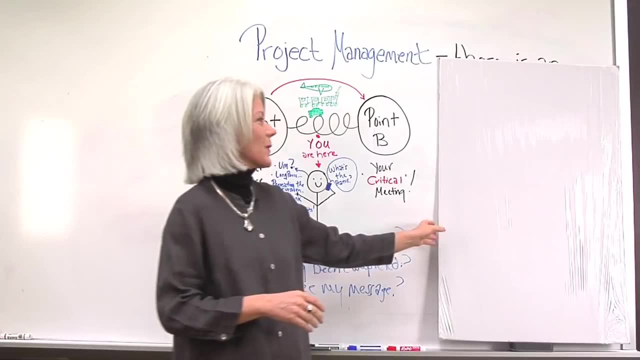 But don't you wish there was an app for that? I know I did So. I told my team, So the team at projectmanagercom has been really busy at work, So I want to unveil to you today that there is an app for that. 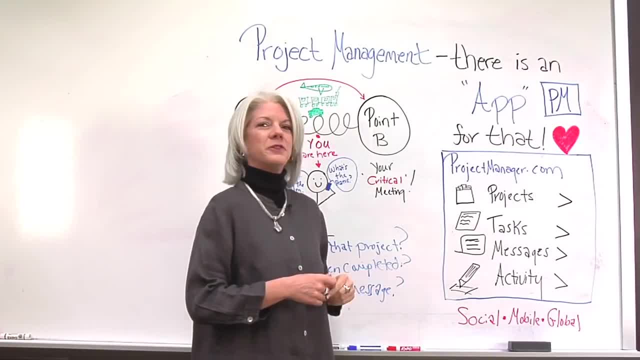 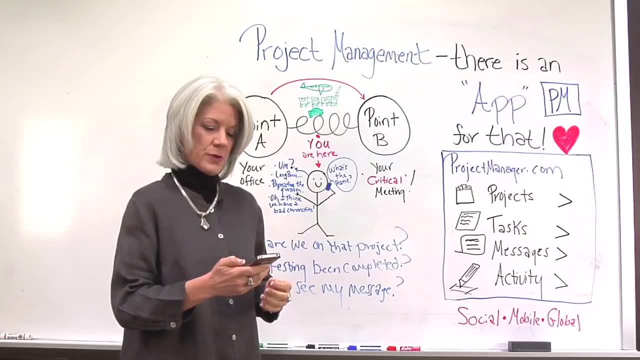 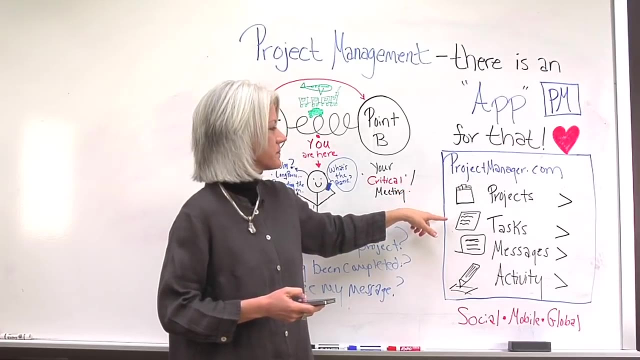 So if you go to your app store you can find the app projectmanagercom And with that app I happen to have an iPhone, so you can pull up your app on your iPhone and actually pull up information On your projects, your task, your messages and activity. 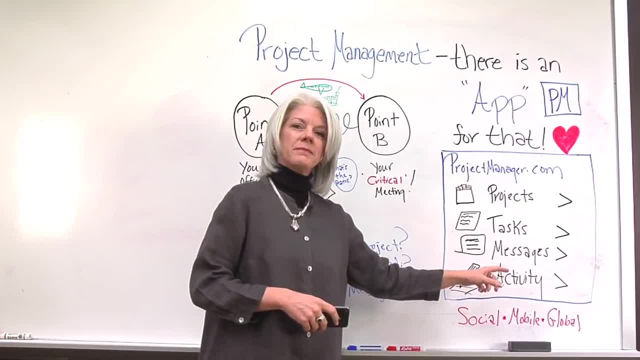 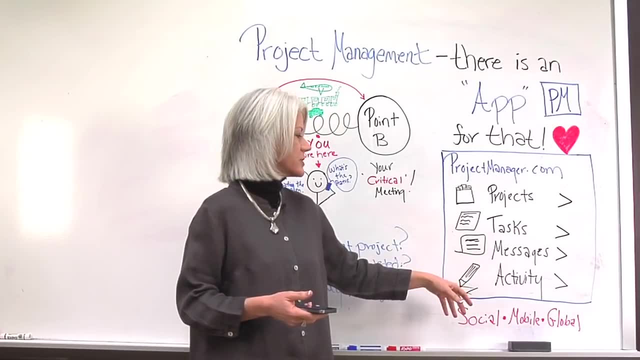 Isn't that cool. That helps me keep social, mobile and global. I can socialize between the members of my team. They can update their task and all of the information. It keeps me mobile. It keeps me going from point A to point B. 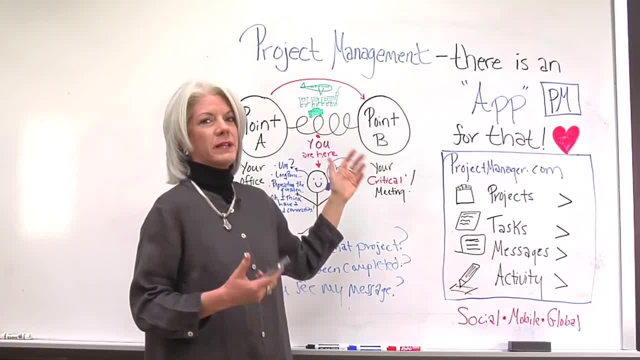 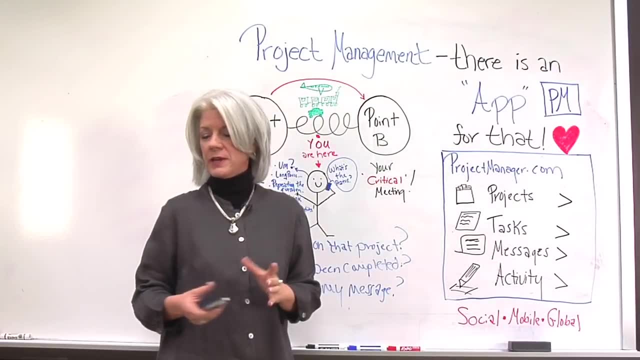 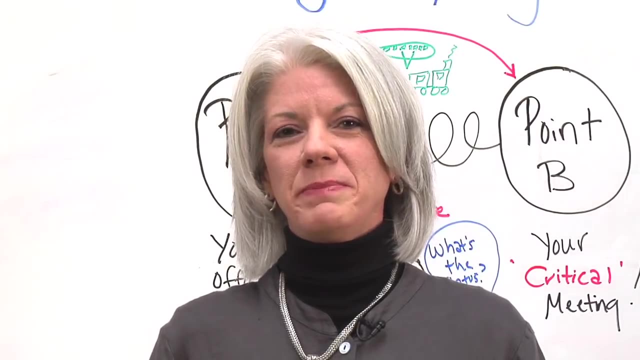 And for my- for me in particular- planes, trains, automobiles- And it enables me to remain global, To get to destinations and and communicate with my team globally. If you're searching for better answers to the questions when you're trying to get to point A, from point A to point B,